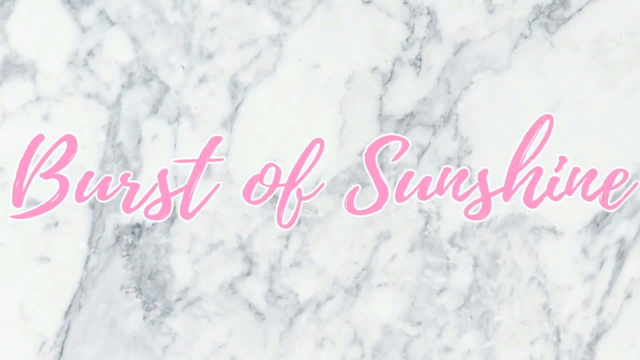 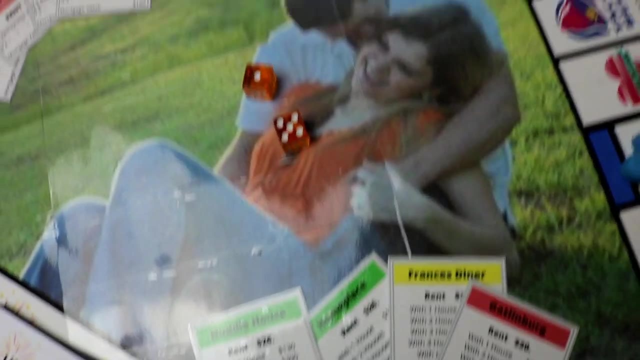 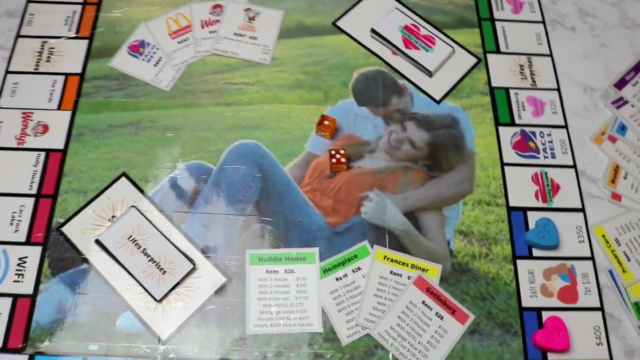 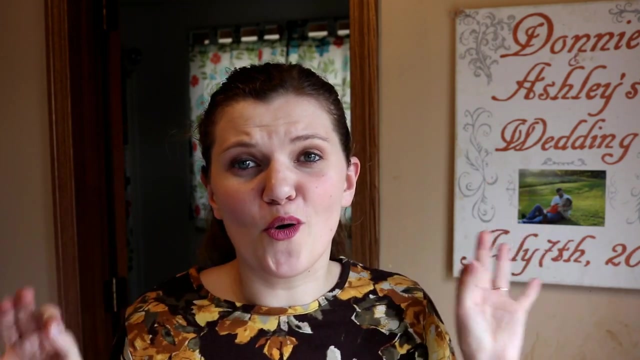 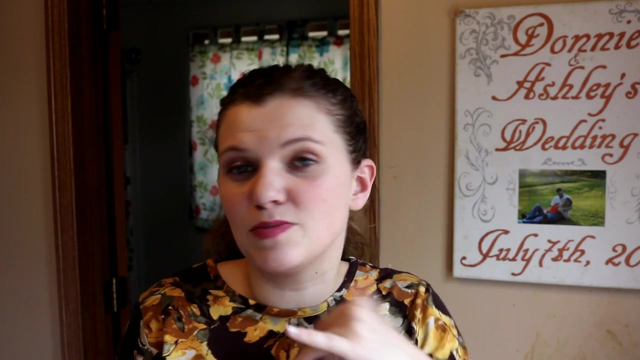 Hey guys and welcome back to my channel, Bursts of Sunshine. It's Ashley. Today I'm going to show you guys how to make your own personalized, custom Monopoly game. Now, this does not have to be a romantic gift. This would be good for just your friends or anyone in your family. 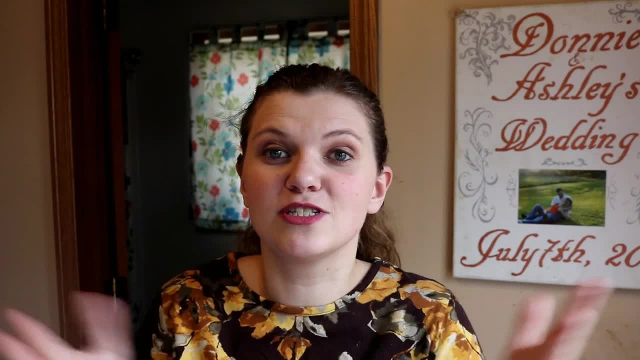 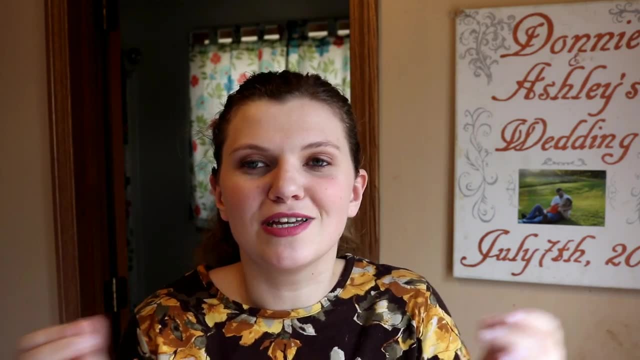 I am using it as a romantic gift, for a Valentine's Day gift for my husband, So I'm going to be calling it Loveopoly. I've seen this on Pinterest a couple of years ago and I thought it was too cute: You can hand make your board on a poster board. I chose not to do that because 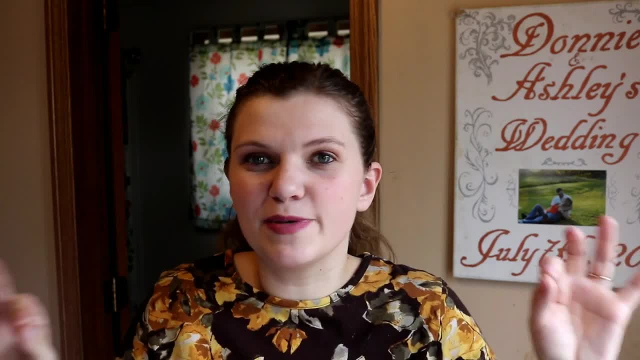 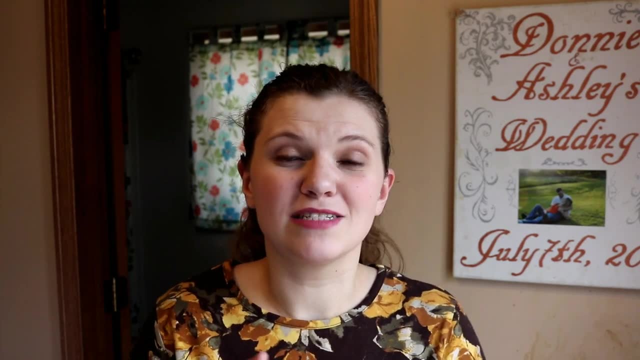 I just wanted to make it digitally and print it out, because that's where I'm a little bit skilled at. I'm pretty good at being crafty on the computer with digital images, So I'm going to show you exactly how I made this Monopoly board. 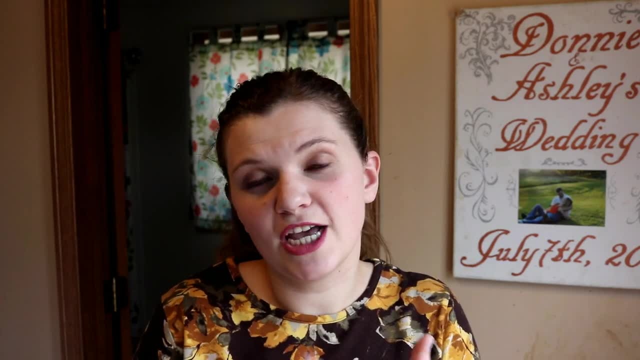 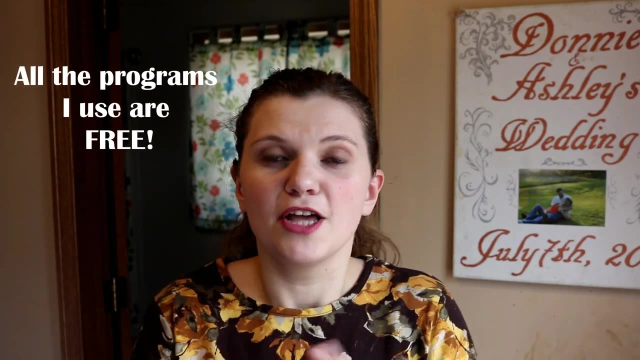 The properties and all the community chests and chance cards and everything strictly on like Canva and Ribbit. That's what I make all mine on, So I'm going to show you guys how I made this board. It's mostly probably going to be me showing you how I use Canva. 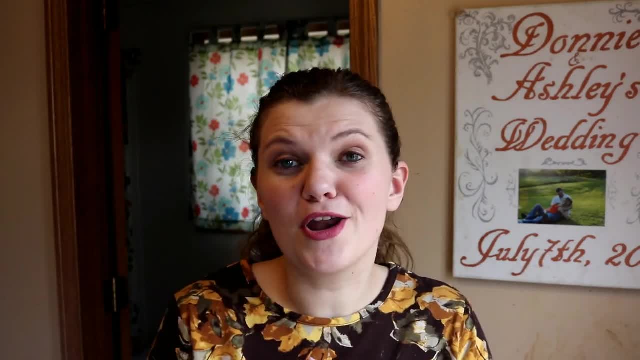 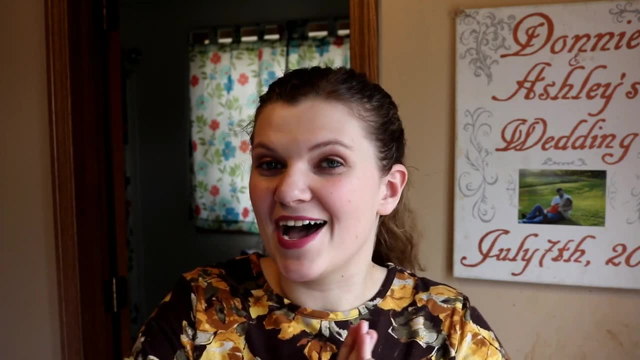 and Ribbit, but it's super easy. I'm going to show you guys how to laminate the board and the properties and cutting out the cards, and how I make my own personalized game pieces. So go ahead and give this video a thumbs up if you like Monopoly. 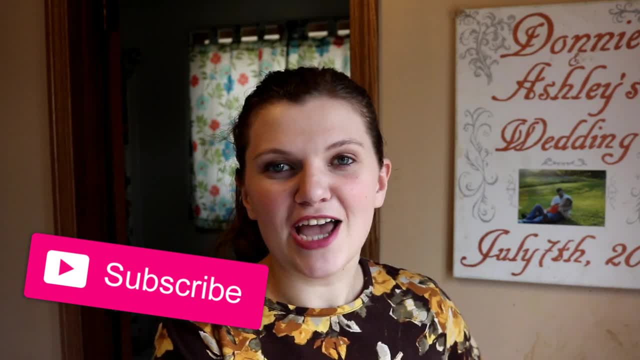 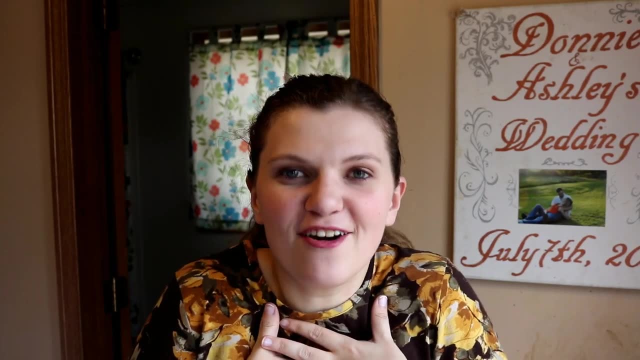 If you're new here, go ahead and subscribe so you can see every time I post a new video. And let's just get into making this Monopoly, because I'm just so obsessed with how it turned out, So let's get into it, shall we? 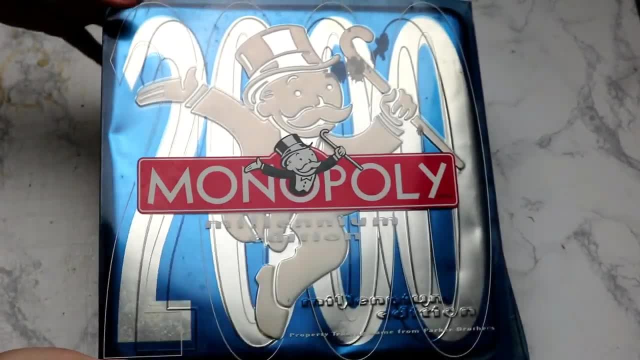 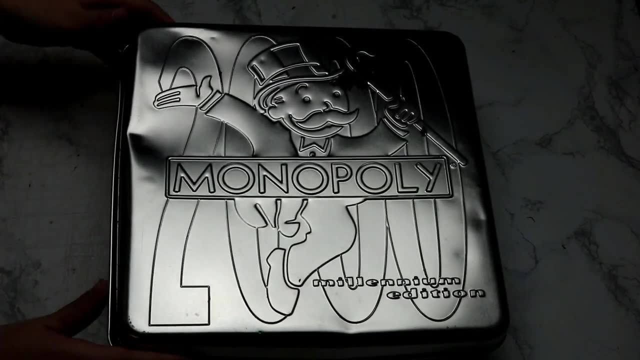 For inspiration. I'm going to be using this old Monopoly game- This is actually from the year 2000- that we haven't touched in years, And so I'm going to use it kind of for my inspiration and so I can see how the cards are set up and how the board is set up And 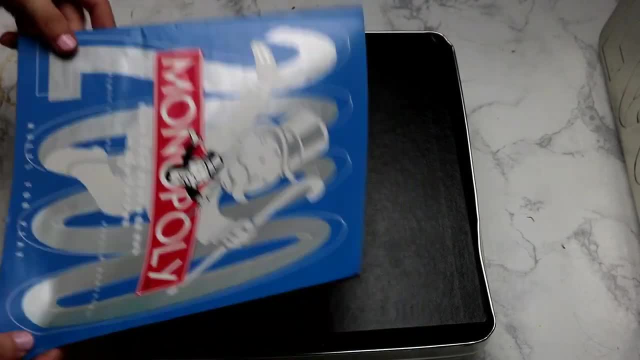 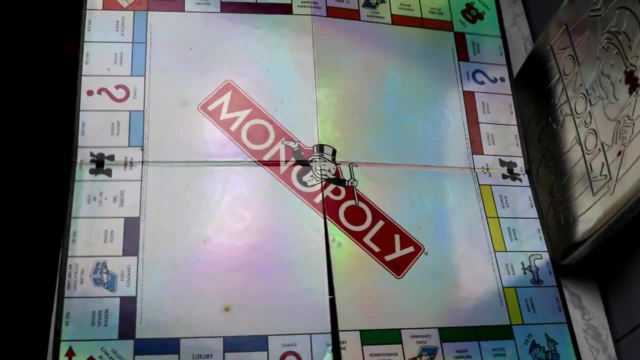 I'm going to make a board out of this game for my game, just so I don't have to make everything. So the board is the first thing I'm going to really take a look at so I can see how it's laid out and the properties, so I can figure out how I want to make my board As. 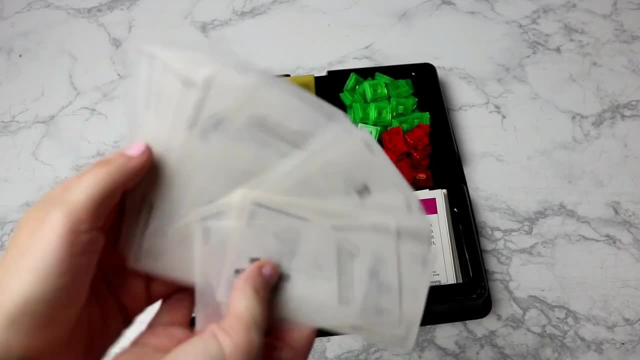 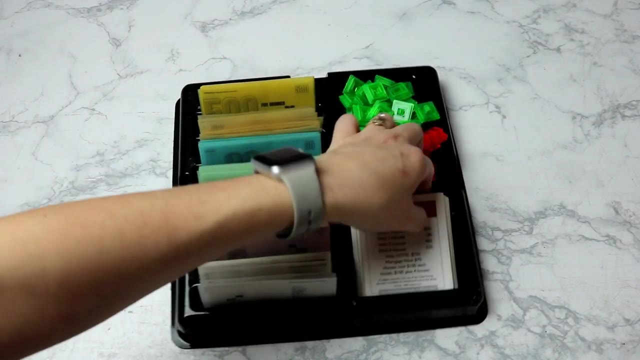 far as the money, I could make my own money, but I feel like that would be really time consuming and waste a lot of ink, So I'm just going to use the money that is here, and also the same with the houses. I could probably make some type of houses, but that would just 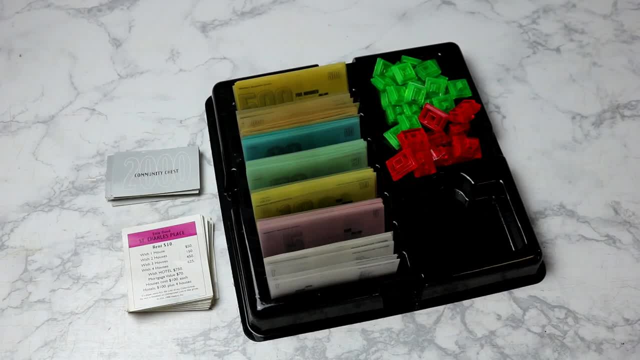 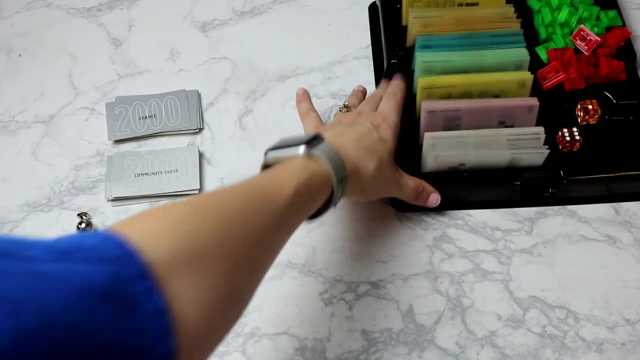 be too time consuming. So I'm going to make the properties, the community chest and the chance cards. Those are the things that we're going to remake for our own little version, And I'm also going to remake the game pieces. So first I save a blank Monopoly board off. 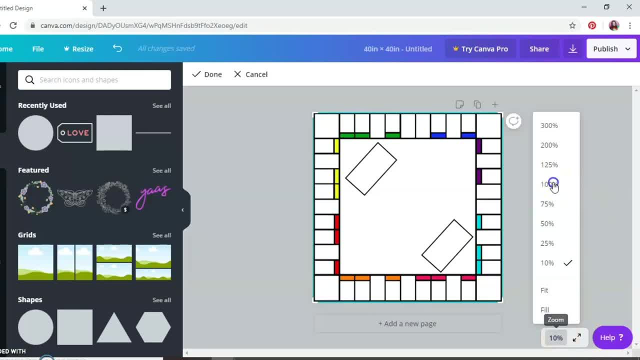 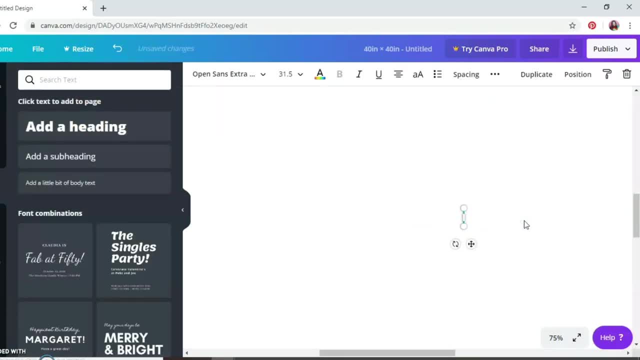 of Google and I open it up in Canva. Original Monopoly board is 20 inches by 20 inches, So keep that in mind when you're making your dimensions on Canva when you're opening it up. So I opened up a blank template of 20 inches by 20 inches, which I always like to. 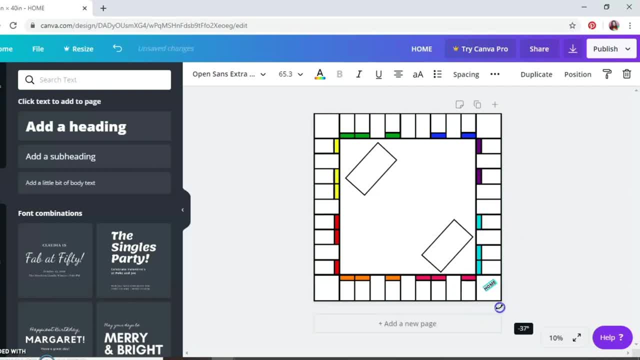 double it, just so I make sure I get good quality. So 40 inches by 40 inches, if you want, And then I have just placed the game board on it so it is the correct size, And then I'm just going to go and make the board. So I'm going to go ahead and make the board And 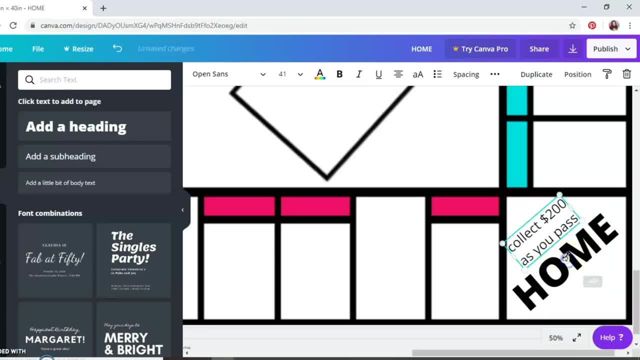 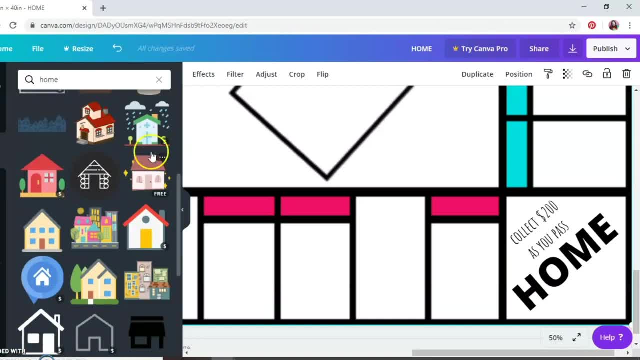 then I'm going to go in and add text and images to kind of customize this how I want it. I'm going to go in and make the home place first, And then I'm going to go in and I'm going to make the utilities and make the properties And I make these all custom to me, You want. 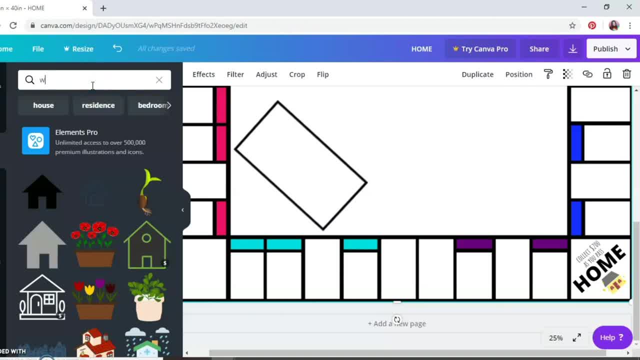 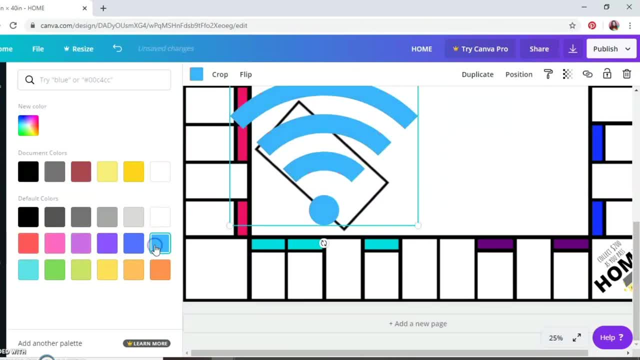 to make these custom to you. So if you're doing this for something with your friends or a significant other or loved one, maybe make all of the properties places you guys like to hang out or places you guys like to go or that's significant to your relationship. 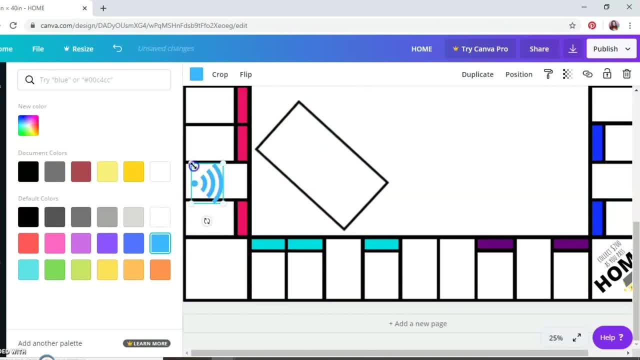 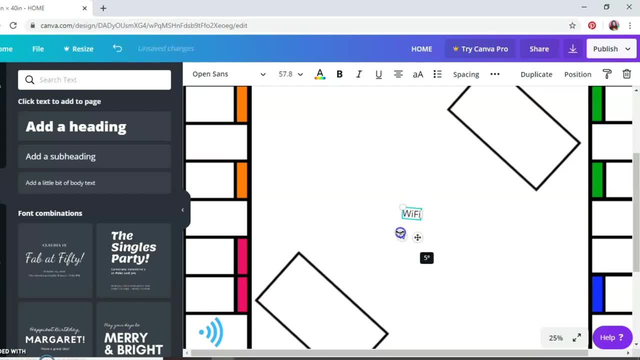 I added in places that are significant to our relationship, into mine. I'm just going to go around the entire board using the text and just naming all of my properties. custom names for us, Of course, make these custom to you, And I'm also going to add the prices. 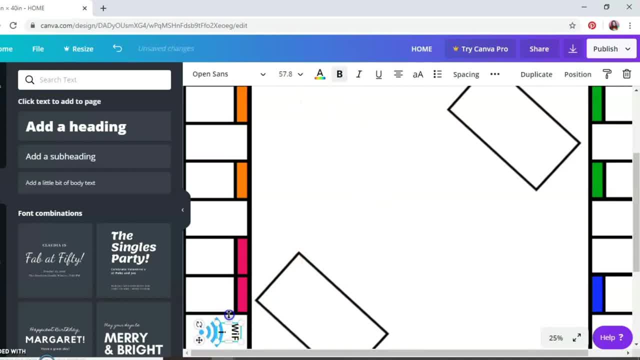 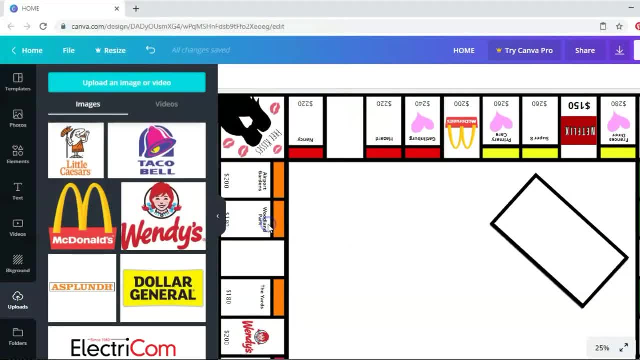 for all the properties as well. Instead of doing the electric company and the water company, I decided to make my utilities Wi-Fi and Netflix. Now I'm just going to show you real quick how I added my image to the middle of this board. So what I did was I just went to upload. 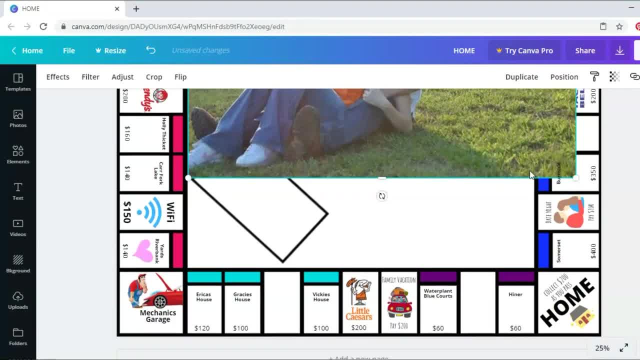 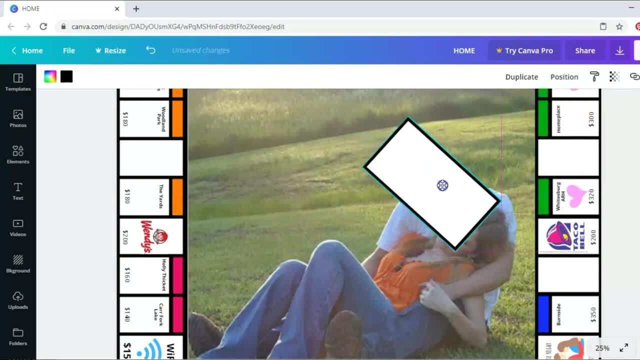 an image and I picked my image I was going to upload. I put it over top and then I just kind of cropped it down so it perfectly fit in the square in the middle And then I used just a rectangular shape to make rectangles for the little cards. the community chest. 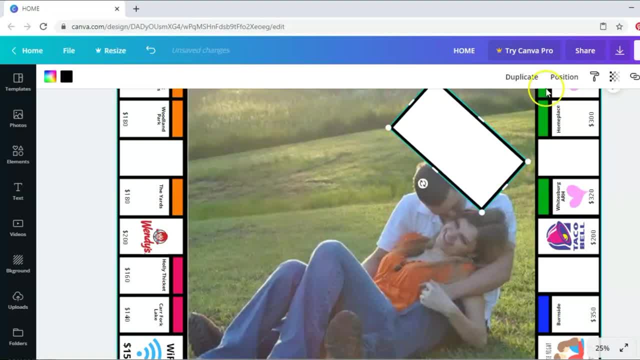 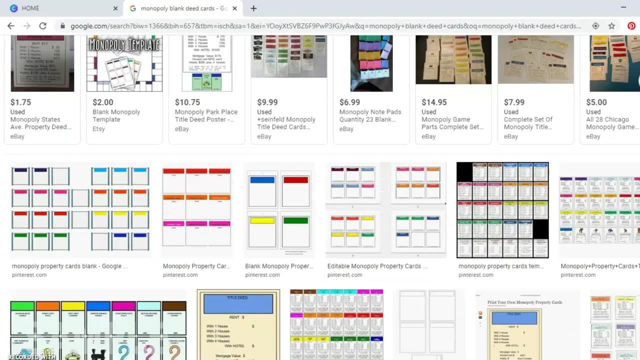 and the chance cards to sit on. So I kind of size them and put them, place them on there on top of the image. Now for the deed cards. for all the properties you make, you need matching deed cards. So I just went on Google and found this blank template for deed cards. 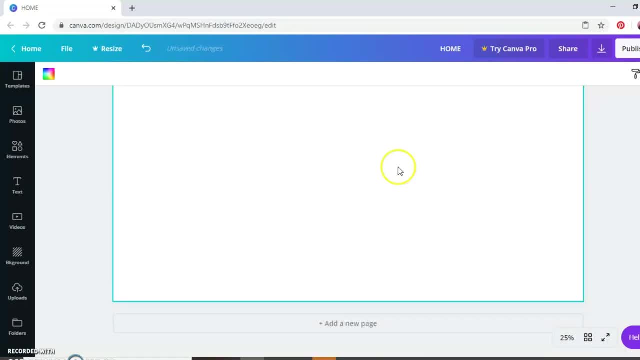 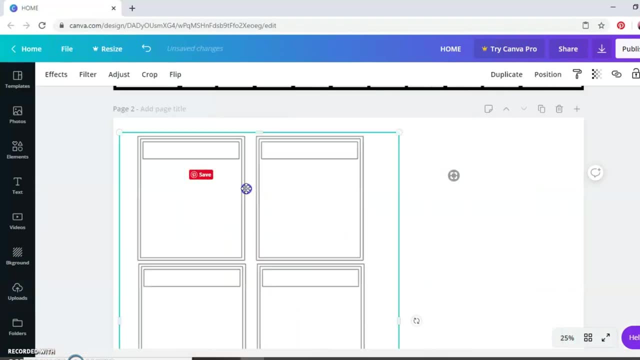 and I added a new page on the bottom of my board here and I just uploaded that image and put it in there. So I did this multiple, multiple times Until I made enough properties to do all of them. And I'm going to show you first how. 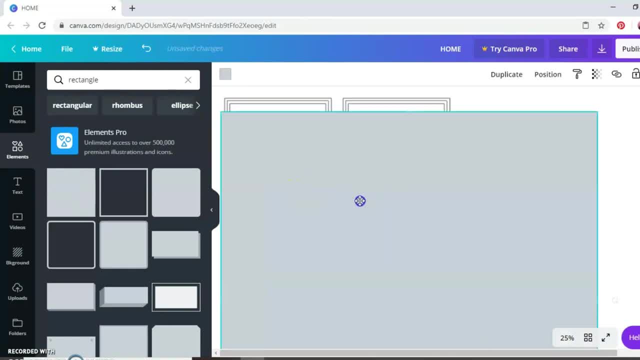 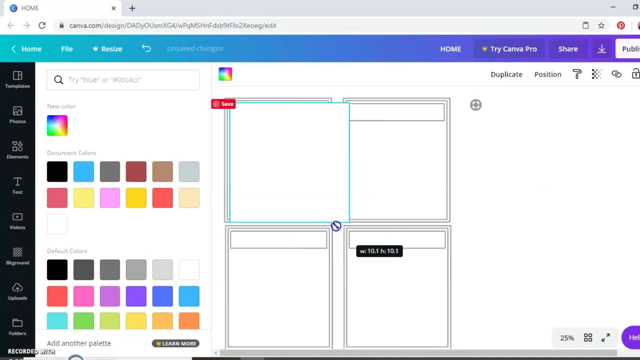 I make the utilities and the restaurants or the railroads. I just did restaurants because that seemed more significant to our relationship than railroads. So I'm going to add a white rectangle first to make these blank cards, So that way they don't have the little rectangles. 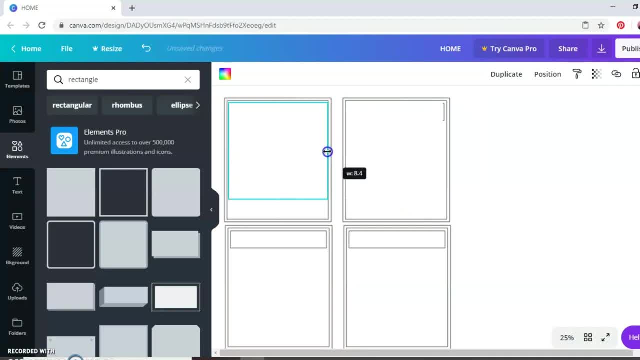 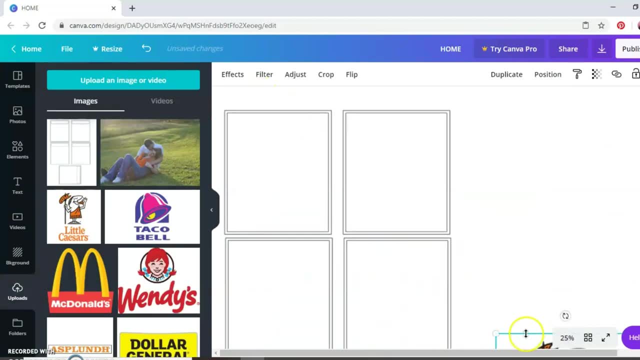 on the top, because the restaurants and the utilities- or sorry, the railroads and the utilities- don't have the little colored triangles. So I did upload logos for different restaurants that I'm going to put in here. These are just restaurants that we like to eat at often or really like his favorite restaurants. 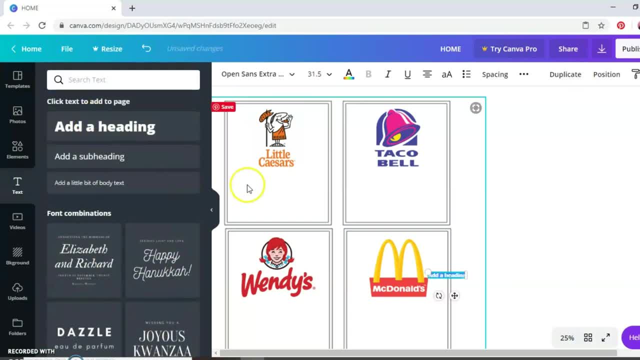 So that's why I chose these. I'm going to add in, of course, how much rent would be if you land on these properties. And then what I did is I sized it the way I wanted it and then I just duplicated it and I put it on each card, so that way they're all exactly. 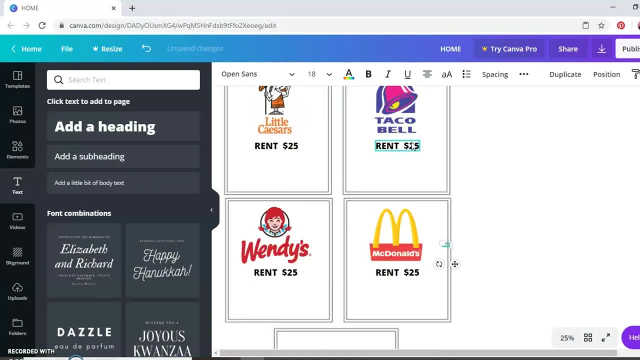 the same size, And then I did the same for the little words that go in it. I actually looked at the cards that I own from my monopoly board to type all these out, but you could probably Google it and get all of the information off of each card, because every property card. 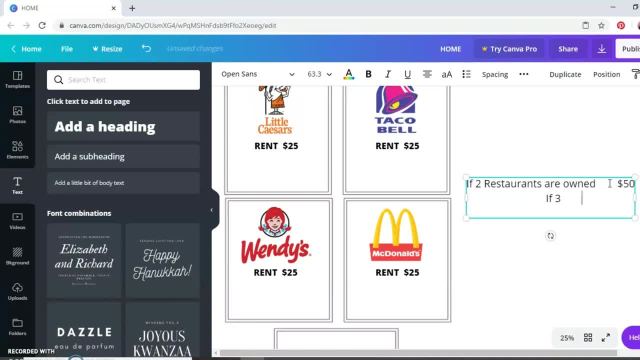 has different prices on them. So I just went in and I kind of just typed it out, what it would say on the card for the. this is for the restaurants or, if you're playing actual monopoly, the railroad. I've seen them done on Pinterest with cruise lines and stuff. 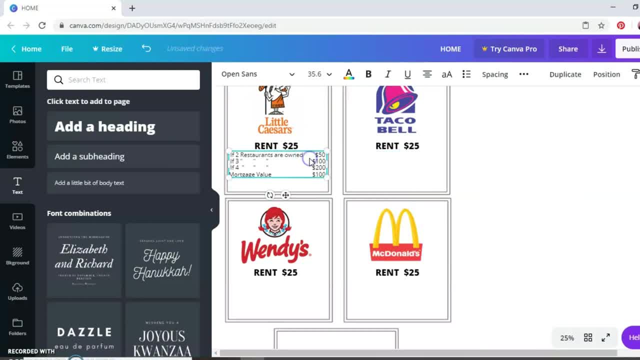 but I just thought the restaurants would be really cute and personal for us. And then, once I have it typed out again, I just hit duplicate, which just copies this image or the print that I have, So that way they're all the same size and they're all lined up. 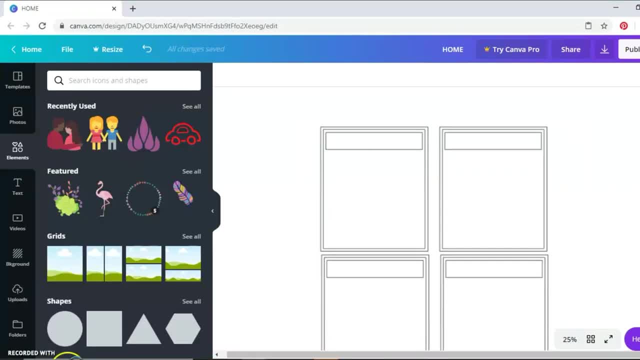 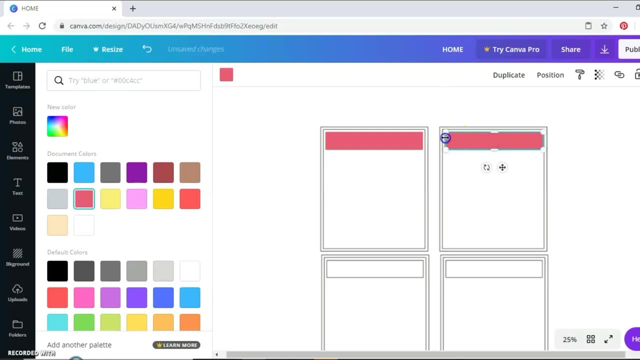 and look perfectly. even Once I get those done, I'm going to show you how I make the properties with the colors. I do the same thing with adding a shape and make it whatever color the property is going to be, And then I just cover up the little white rectangle. 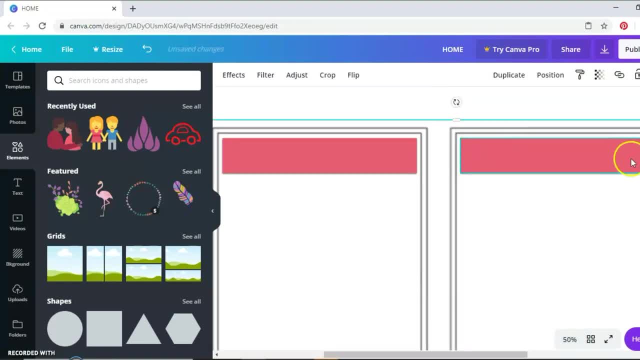 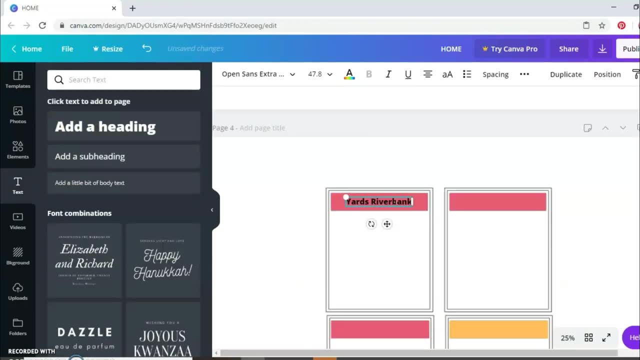 with it. I kind of had to zoom in to get it to fit perfectly, because sometimes it don't always just match up right. Then I'm going to go and add the text and I'm just going to type in the locations. As you can see, I already have a few of them done. when I recorded 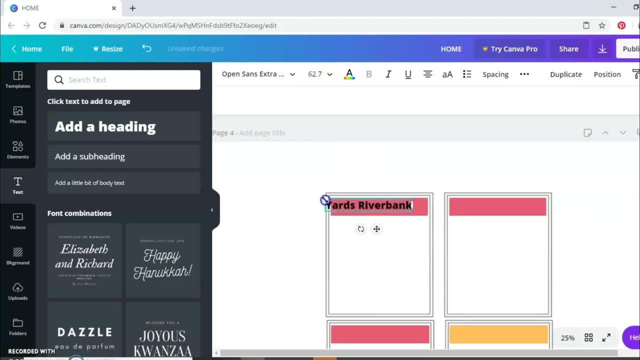 this, but it's because it would have took me a hundred years if I'd recorded every single step. So then I went in and I added my words, I duplicated it, So it's the same font and same size, And then I would just change what it said until 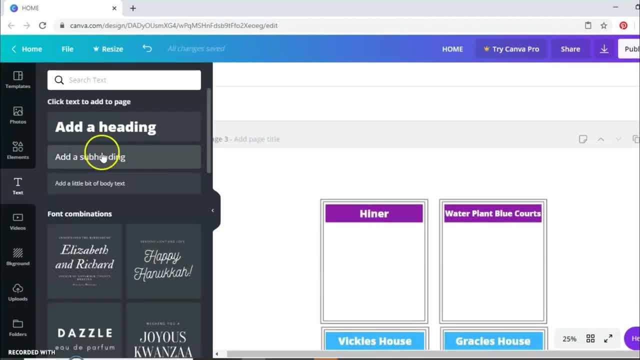 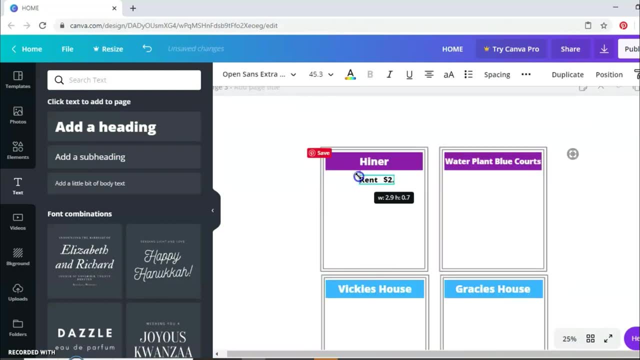 I got all of it, All of my properties named. Then I went in and, of course, added my rent, sized it the way I wanted it, duplicated it and then put it on all of the cards. So they all had the rent amounts And of course I changed them based on the cards and I priced these exactly. 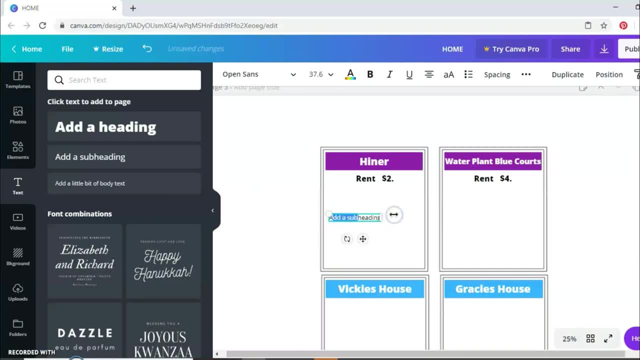 as they're priced in regular Monopoly. The only difference is I just changed the name of the properties. So I did go in for every single property and I changed the prices on every one of them to match what they are in the original Monopoly game. You can totally 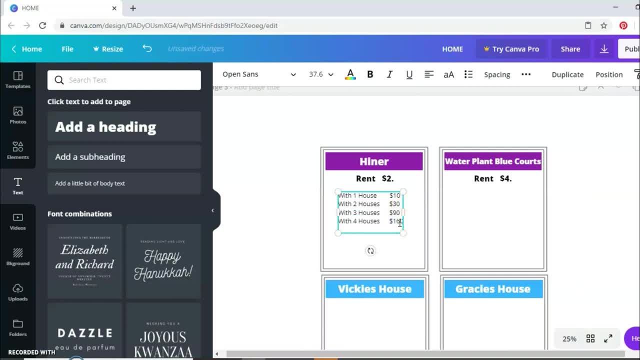 price these however you want. I just wanted it to make it So. it was playable, just like regular Monopoly, because Donnie loves Monopoly- Donnie's my husband, by the way, if you didn't know. He loves Monopoly and we do play Monopoly sometimes. 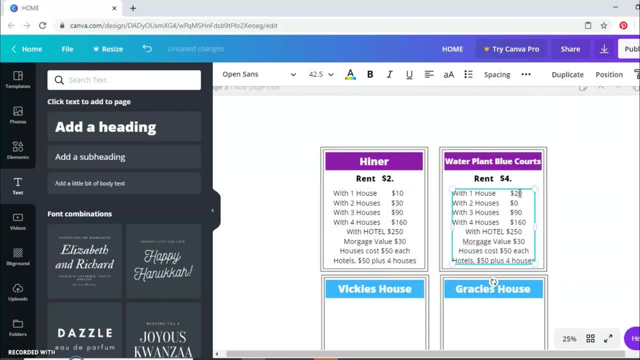 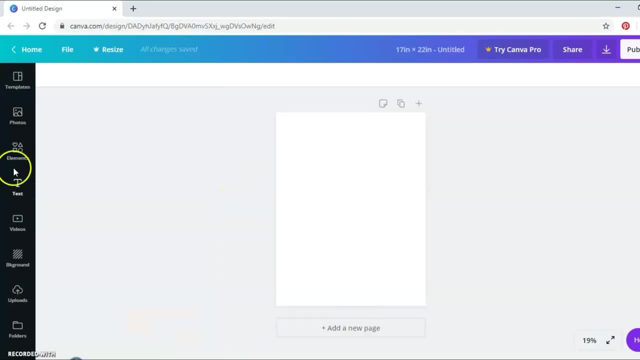 So I just wanted it to be very playable because I really think he's going to enjoy it if he can actually play it, because he likes to beat me at Monopoly. So I just did this for all of the property cards until they were all priced and made up. Now I'm going to open. 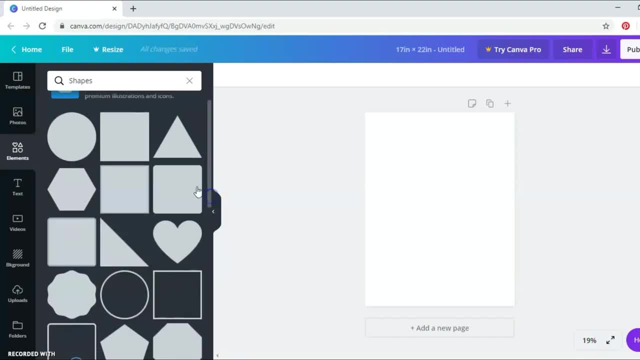 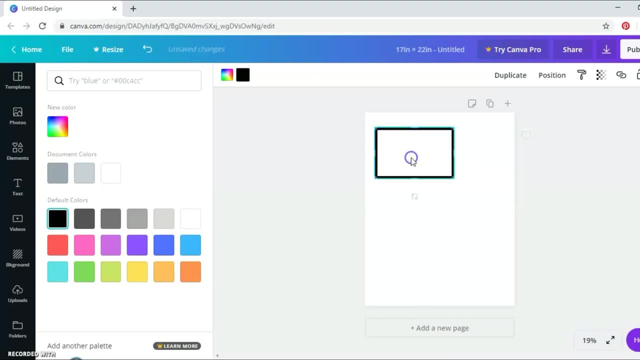 a new document and this is just going to be the size of a sheet of paper, So eight and a half by 11.. I'm going to use this to make my community sheet. I'm going to use this to make my community chest and chance card. So I'm just going to add a rectangle and I'm going to use the 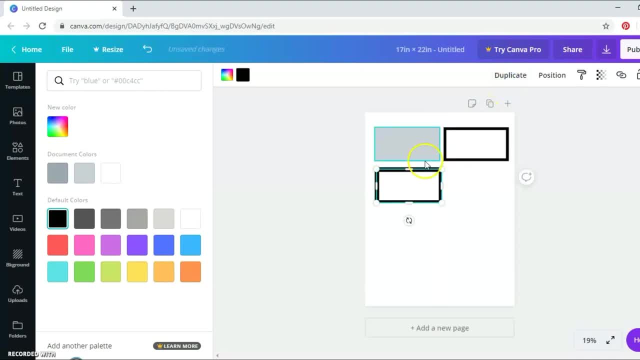 one with an outline, so that way I can see where to cut it out. And then I'm going to size it down about how. about a rough estimate of size? I want it. I don't know exactly how big I made these cards, I just kind of eyeballed it. So about eight would fit on a sheet, and 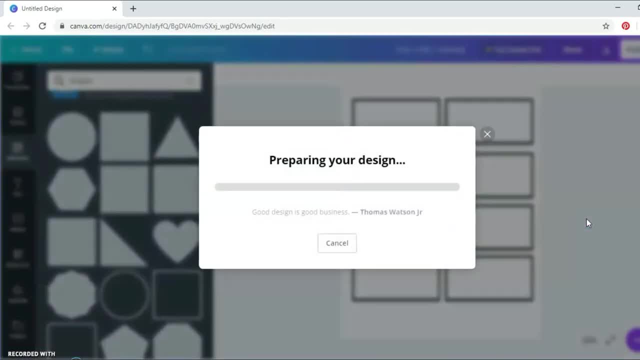 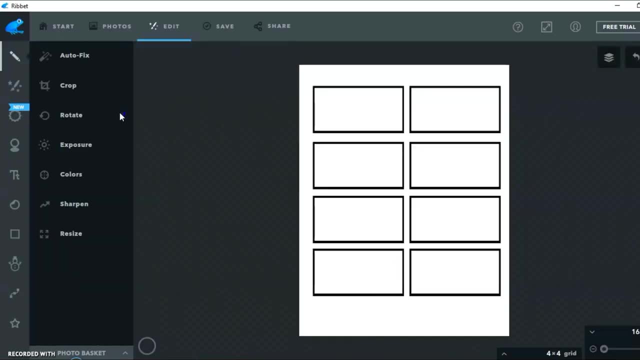 then I duplicated it So they all, of course, were identical, And then this is going to be my layout for all my chance and community chest cards. So the first thing I did was save this, So I have this exact layout, and then I open it and rib it And the reason. 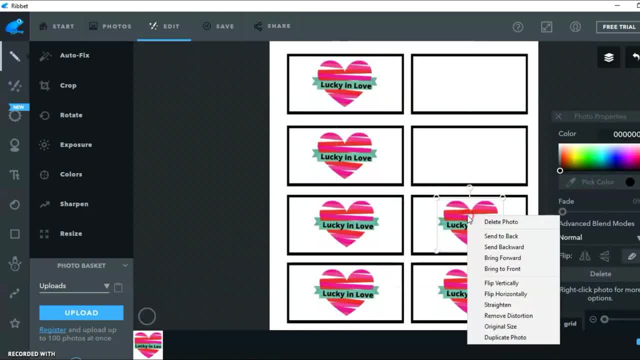 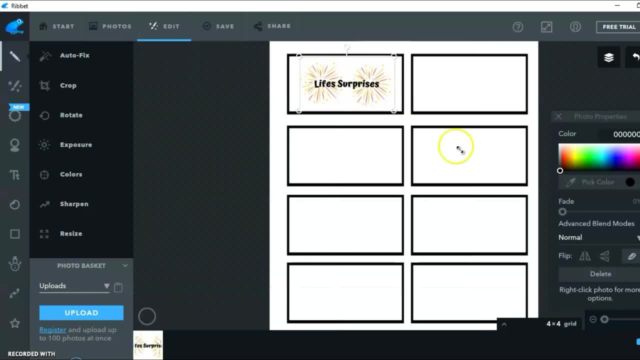 I did this is because I want each of these to print out the exact size- Same size- So I use the same image for all of them. So first I made my logos for the back of the cards and then I deleted them and use the same original image to add the. 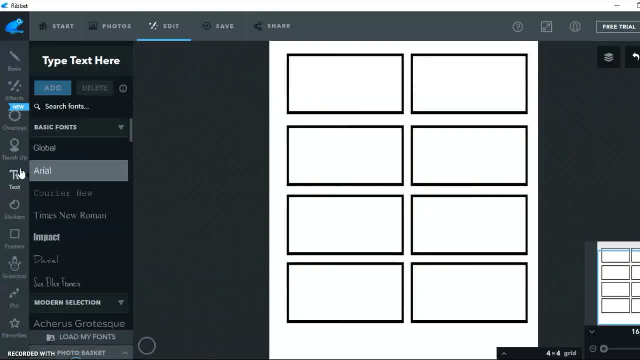 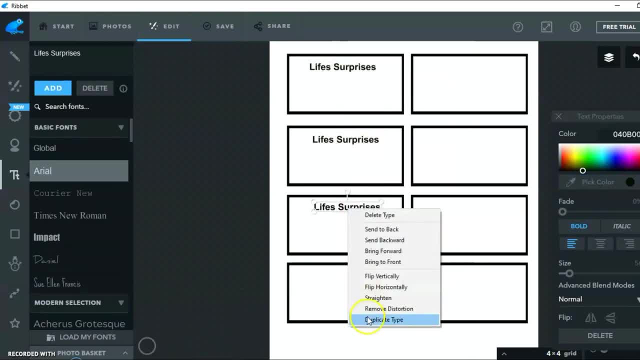 logos for the other cards, just so they're all exactly the same size. After I made the images for the backs of the cards, I went back in, deleted the images and, using the same photo, I added all of my little random activities is the word I'm going to use, Like. 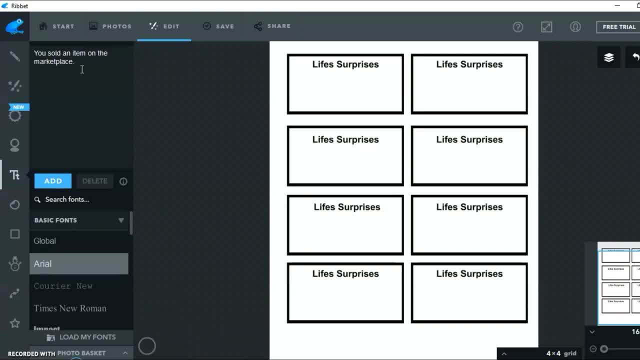 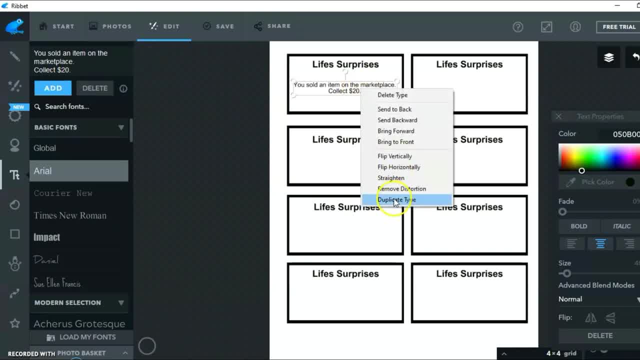 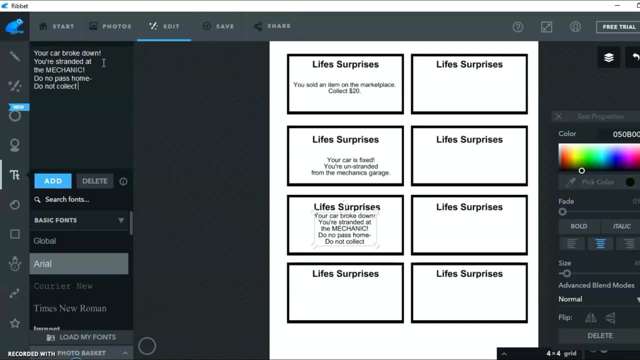 game you like. i added some that are like: go on a date night. i added some that's like: go to, uh, the huddle house and eat, collect 200 if you pass home. you broke a phone charger, replace it, pay 15, like. just things that seemed like they were relevant. so, yeah, definitely customize this to your game. 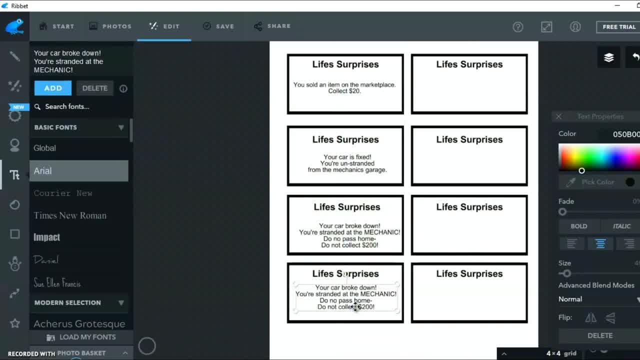 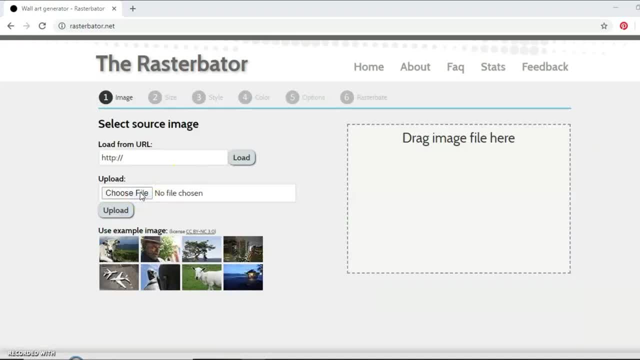 and to whoever you're making it for, because it will make it so much more fun. so next i'm going to make my monopoly board, where it's printable on multiple sheets. so i got to this website, rasturbatornet. i don't even know how i found this website. i come across it many years ago. 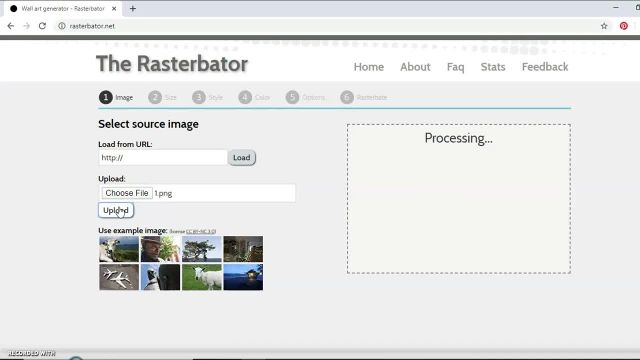 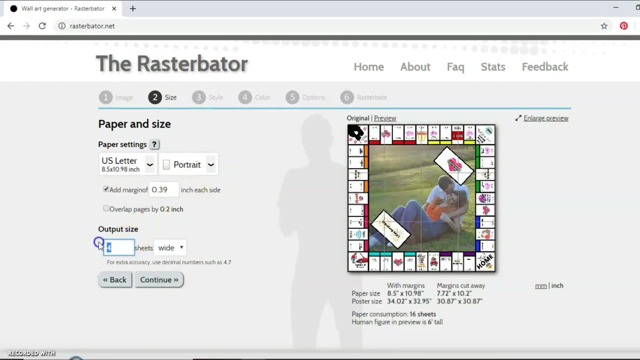 when i was doing wood projects and i'm going to upload the image of my monopoly game board. so on this website, of course, change this to us letter. if that's the size sheets you're using, you can change your board out so you can print it as big as you want on how ever many sheets you? 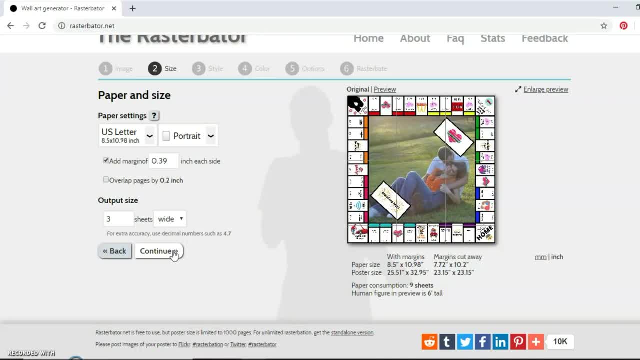 want. i'm going to do three sheets wide and i can tell you this actually come out to be larger than 20 inches, um, so just keep that in mind. it is going to be about three or four inches larger than 20 inches, if you want it to be larger than 20 inches. if you want it to be larger than 20 inches, if you. 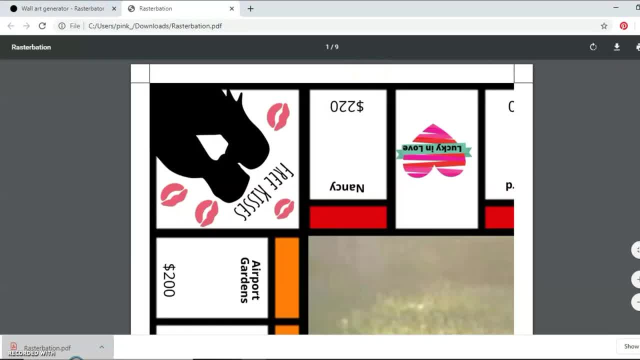 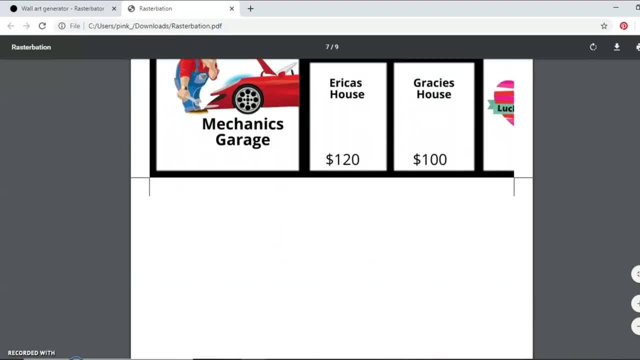 do the three page one like i did. it makes your image into a pdf file that can be printable and then taped together into like one big poster, which is what i wanted, and this is completely free to use. all the programs i'm using in this video are free to use. then i'm going to print out my board. 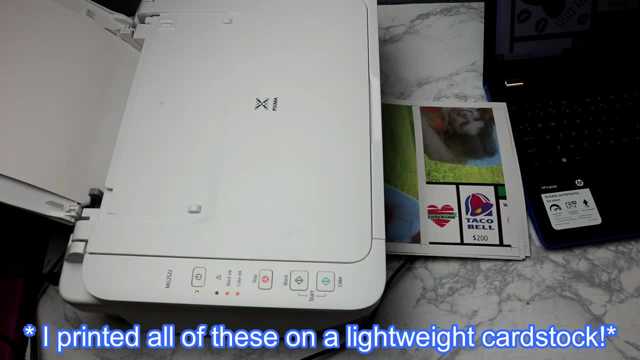 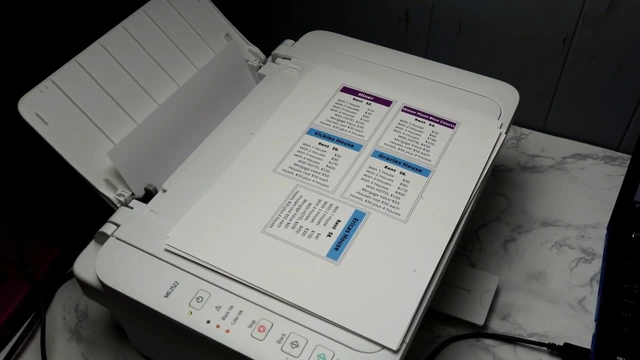 and print out my properties and print out my chance and community chess cards that i've made, since i now have everything made up. so to print out the chance and community chess, first i print out the words and then i put the same piece of paper back in the printer so it prints on the 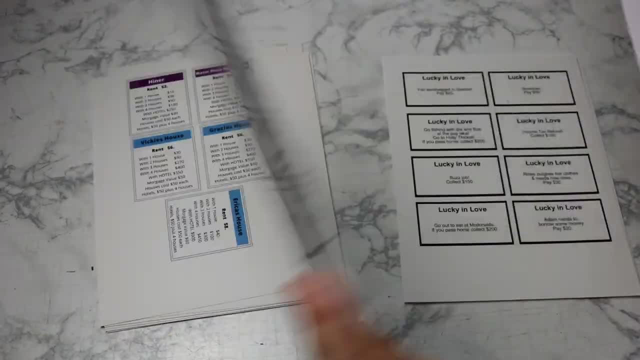 other side of the sheet and i print the logos. so i'm going to print this out on the other side of the sheet and i print the logos. so if you so that way they perfectly print out on the cards evenly, just like on the real game where you've got. 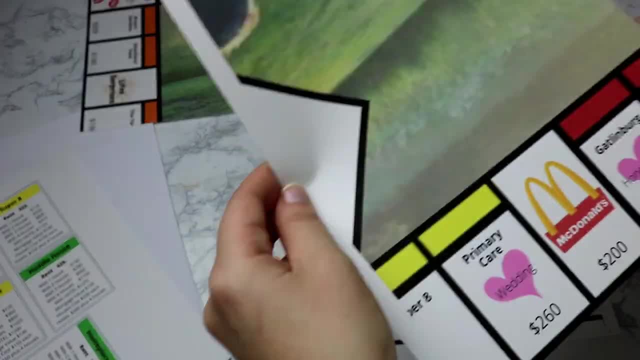 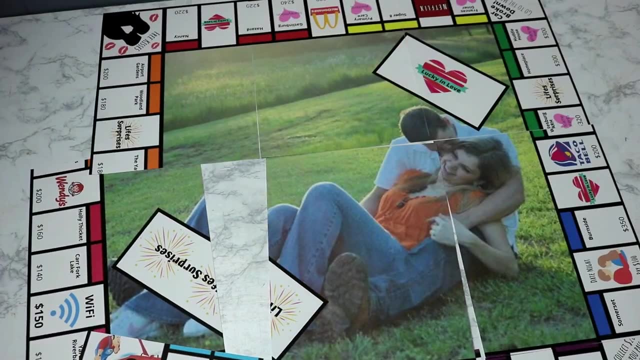 a front and a back. now i'm going to take scissors and i'm going to trim off all of the extra margins off of my game board and place it together so it looks beautiful. and then i'm going to add some scotch tape just a little bit here and there, just to kind of hold it together so i can laminate it. 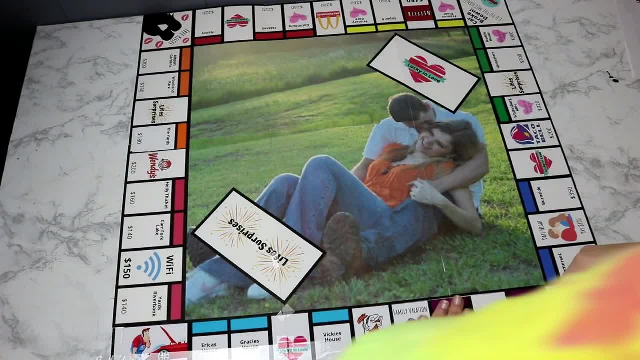 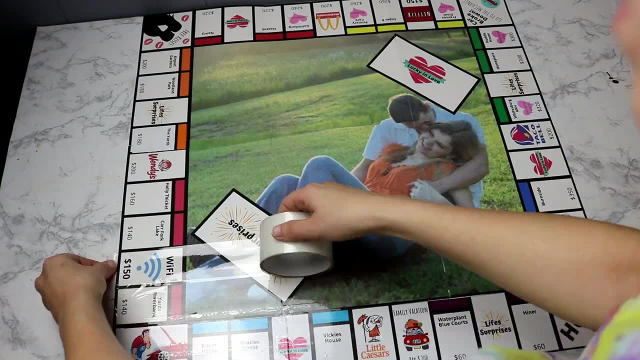 so i don't have a laminator. if you do, i mean, jesus- that will make this so much easier. i do not, so i'm going to use my old, handy, trusty packaging tape. so what i'm going to do is i'm just going to lay the board out and then slowly tape over the entire length of the board, and then i'm 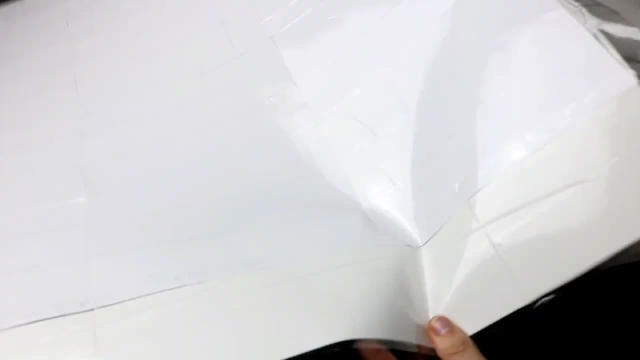 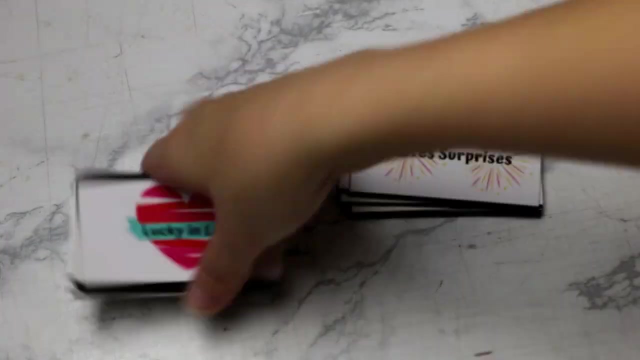 going to flip it over and tape over the entire length of the board again, of course leaving a little excess on the edge so it kind of seals it in, and then i'm just going to take some scissors and trim off my excess. you will get a few wrinkles in this when you're doing it. just rub them out. 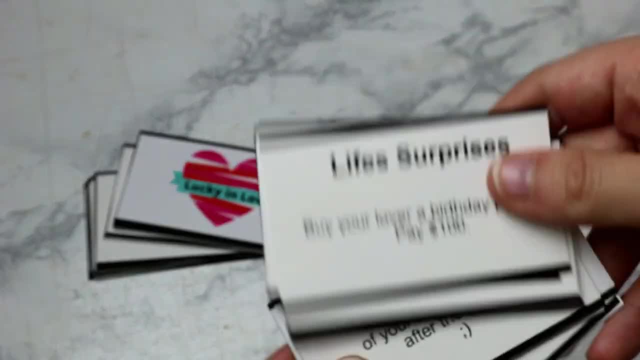 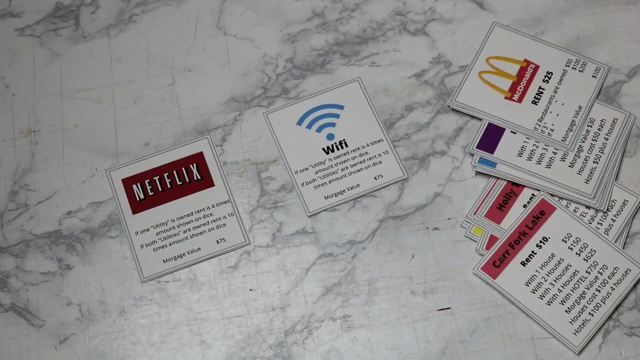 with your finger. it's fine. i cut out all of my little cards for my life, surprises and lucky in love- which is my chance- and community chest cards, and for storing i just wrap a rubber band around them. i'm going to also laminate my property, these and my utilities, just so they're a little bit sturdier. i did not laminate the chance and 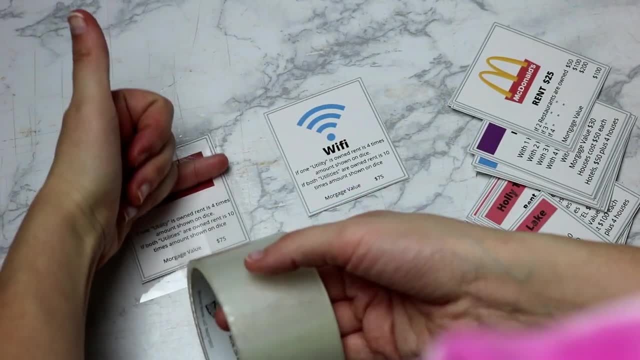 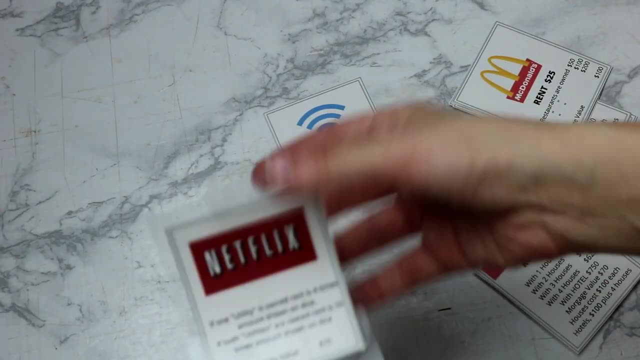 community chest cards. but i'm going to laminate these and it's the same process: just put some tape on it so it overhangs off the edge, press it down so it's on there good and flat and sealed, and then i'm going to flip it over and do the same thing on the back again if there's wrinkles. just 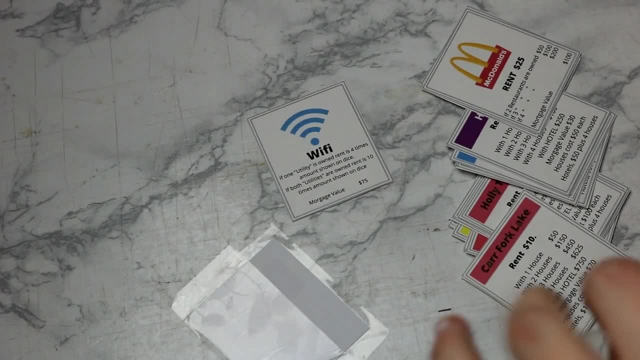 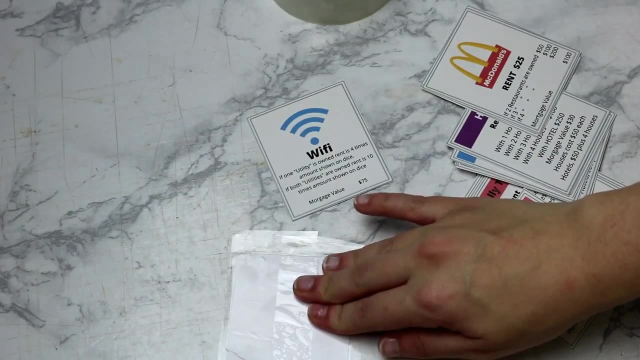 kind of rub them out with your finger. just try to lay it as flat as possible and you shouldn't have too many problems. nobody's going to notice a few wrinkles here and there, so i'm going to press all the tape down. really good, so it's nice and secure and sealed. 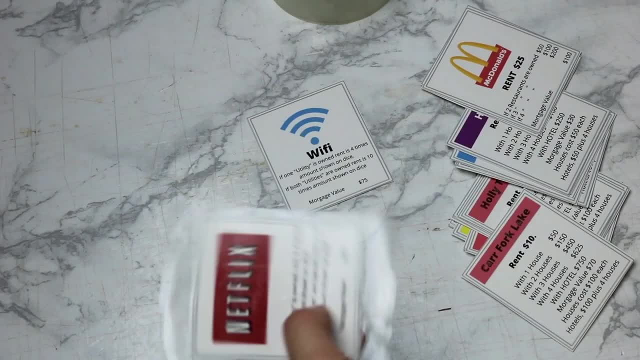 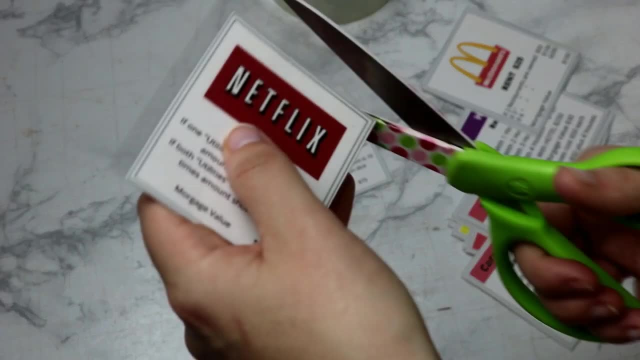 then i'm going to take some scissors and i'm going to trim off the edges, all of the excess tape right along the edge of the paper, and, as you can see, it laminates it. and i did this for all of the properties and all of the utilities. 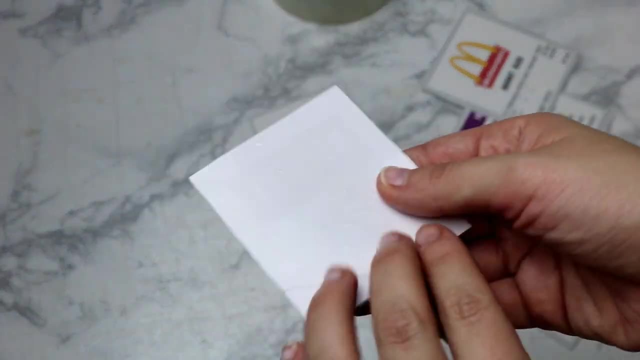 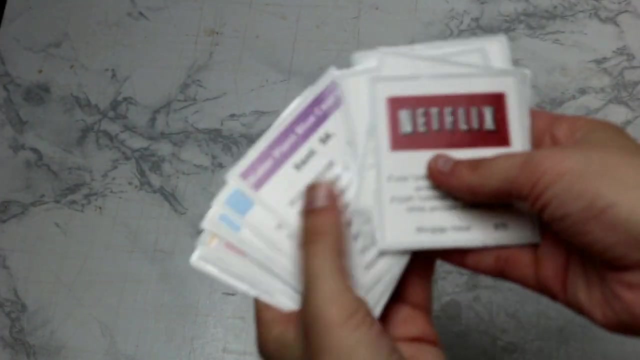 oh, let let me mention, by the way, i use cardstock for all of this. i printed every single thing i printed. i printed it all in cardstock, so it's not regular paper. it's just a little bit thicker than regular paper, so keep that in mind too. i definitely. 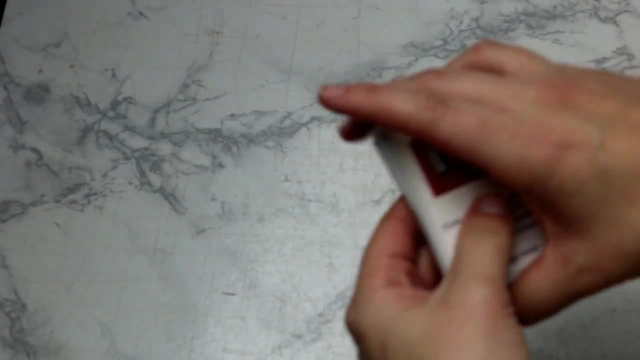 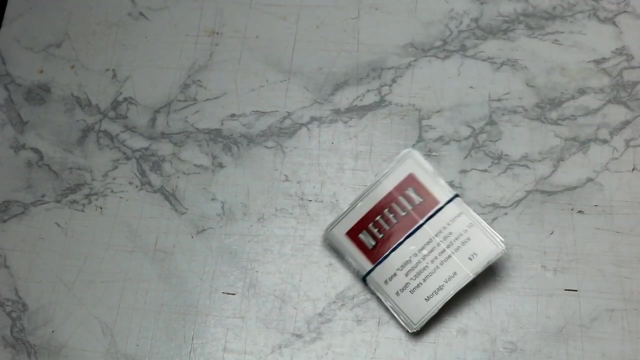 use cardstock and not thin flozy paper. i feel like that that matters. so again, once i get all these laminated, i'm going to put a rubber band around them to store them, and they're ready to rock and roll. we have to have some custom game pieces. i don't want to use the crappy ones that 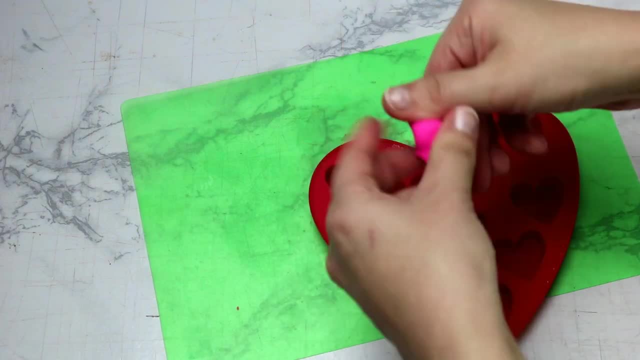 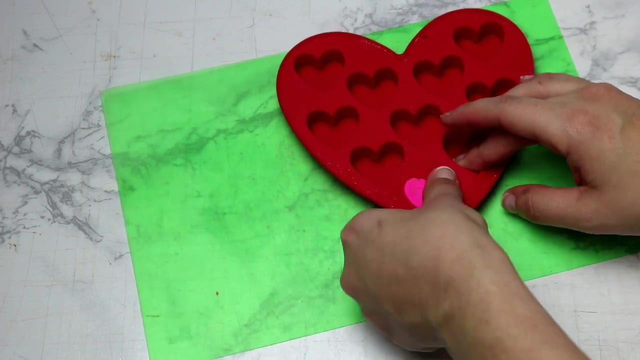 my monopoly comes with because, frankly, my monopoly does not have any cool pieces. so i have this little heart mold that i got at the dollar store for a dollar and i'm going to just take some polymer clay, some of the oven baked polymer clay. you can get this at the dollar store, walmart craft. 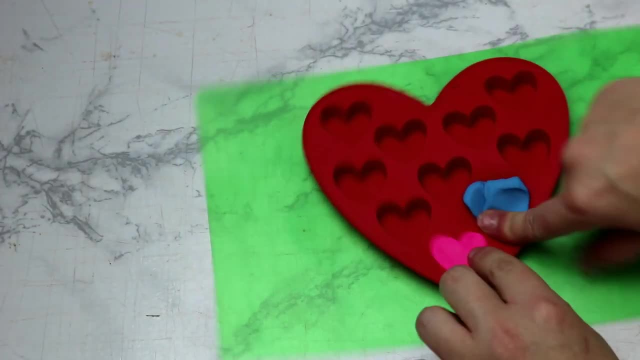 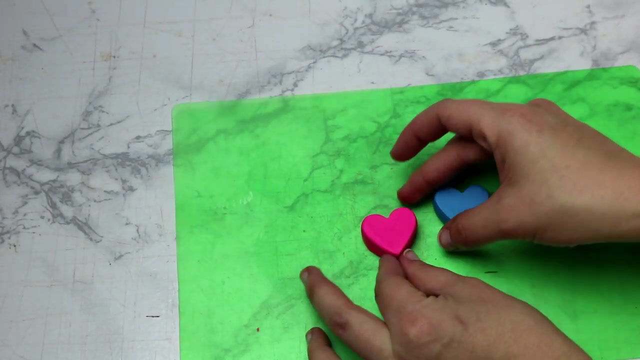 stores and it's super cheap and i'm just going to fill up the heart. i'm going to do a blue one and a pink one, just one for him and one for me, and you can do these whatever colors or shapes you want, and i have these little letter presses i'm going to use. 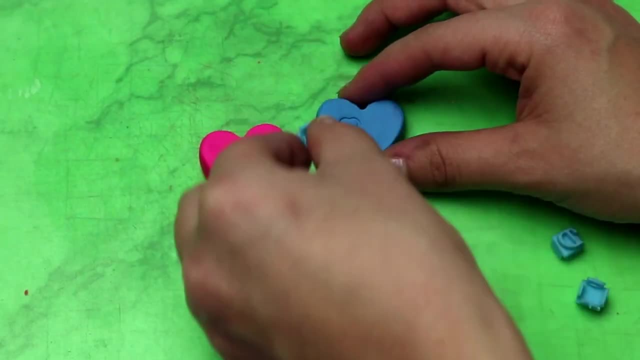 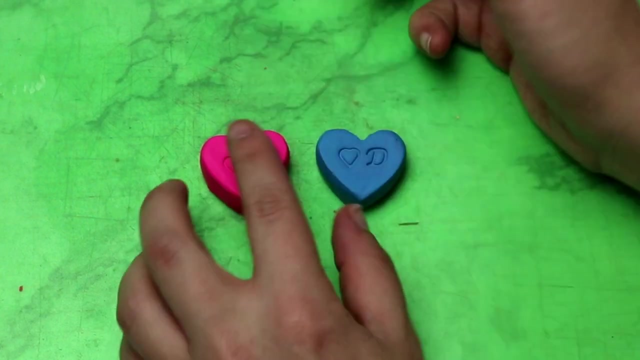 just to kind of customize them a little more. and i'm going to put a d on his for donnie and then, of course, an a on mine for ashley, and i'm just going to press it in there with my fingers. it ain't. no, it don't have to be professional, because it's just for my little loved one here and i'm 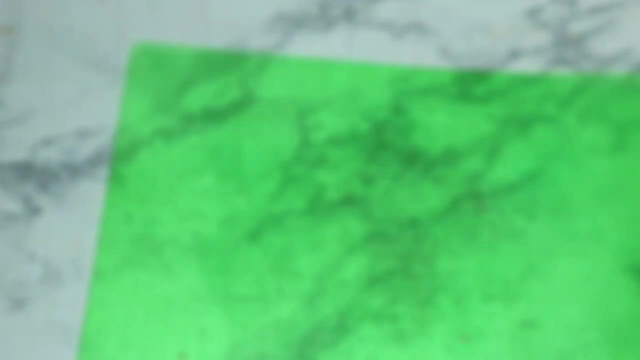 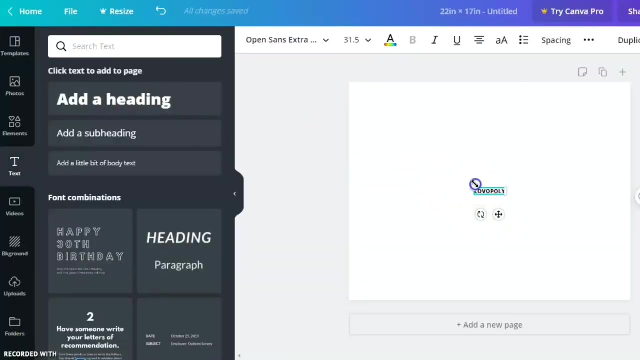 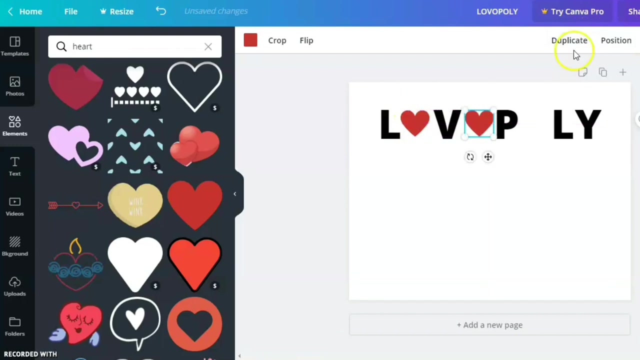 going to bake these in the oven according to package instructions, so they are sturdy. now i'm going to make an image for the inside of my box, because i'm going to store these in a wooden box for donnie, just to kind of present it to him in, and so i did just open up a standard size sheet of paper on. 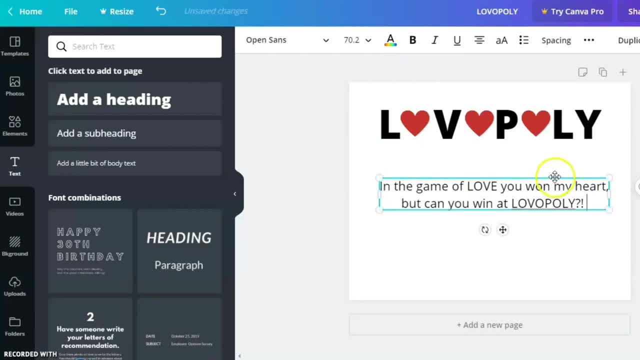 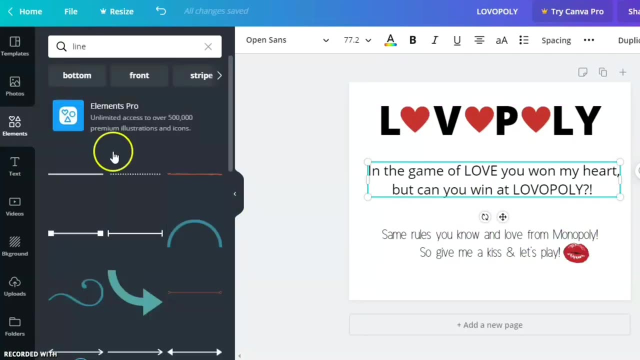 canva and i'm just going to kind of customize my own little message, just letting him know what it is and how to play composite to see what i'm doing, if you want. i just went in and added text and images and scooted them around until they looked the way i wanted them to. a lot of valentine's day. 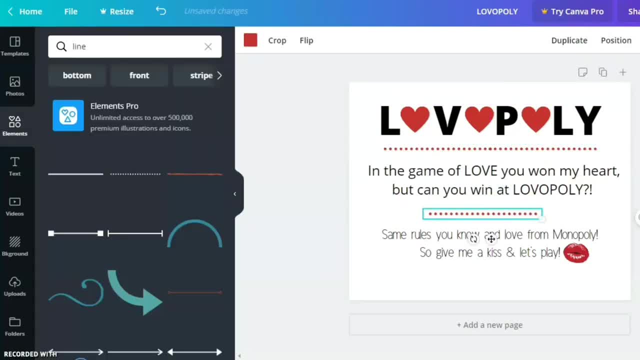 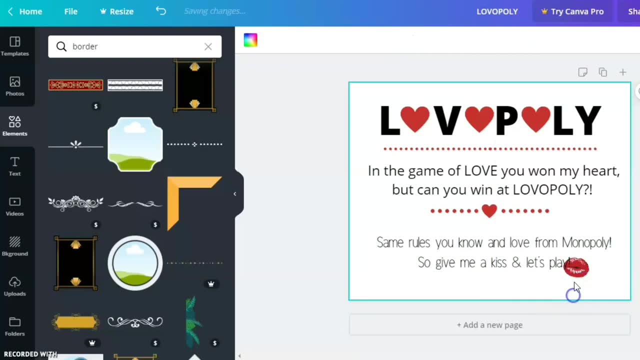 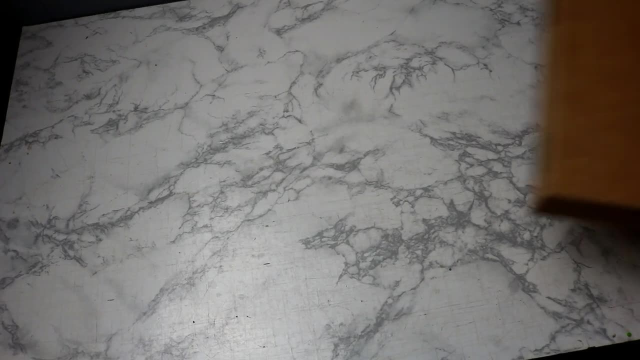 ish looking colors, added some hearts and some lips and just some cute messages, and i just kind of adjusted it here and there until i got it looking how i wanted it to look, and then i did just print this on regular paper. so now i'm going to take my wooden box. 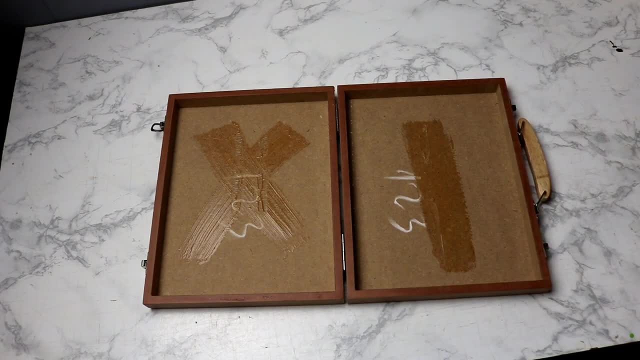 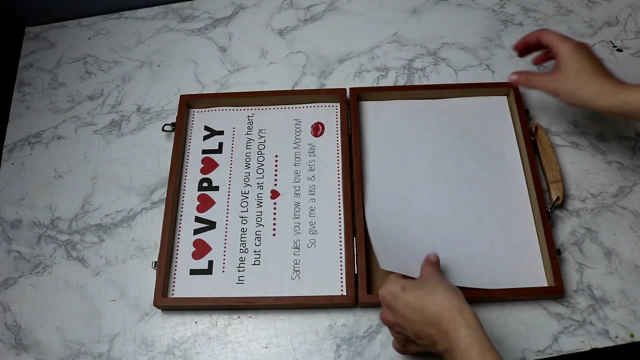 you can get wooden boxes at tons of places. this actually was a cheap art set that comes from the dollar store. I just took the art supplies out and i had an empty box. i'm going to add just a blank piece of paper on the bottom and my little instructional paper on the top, and we not only'll be able to punch it out, 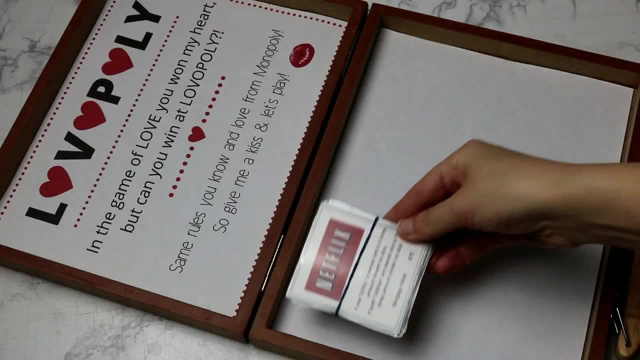 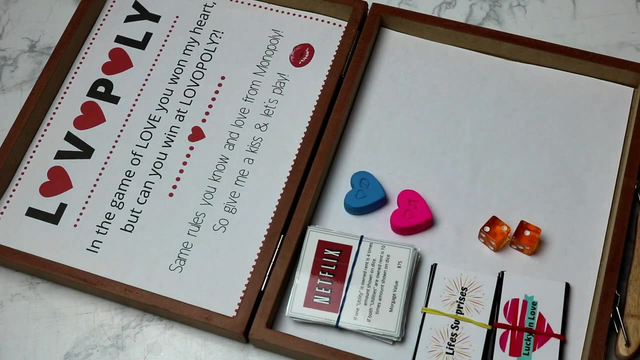 we have a personalized little box for air pieces. So I'm going to add in my properties, my chance cards, my game pieces, and then I'm going to throw in the dice and money from my other Monopoly game and also some houses and hotels, just to kind of make it look complete. And then we have our 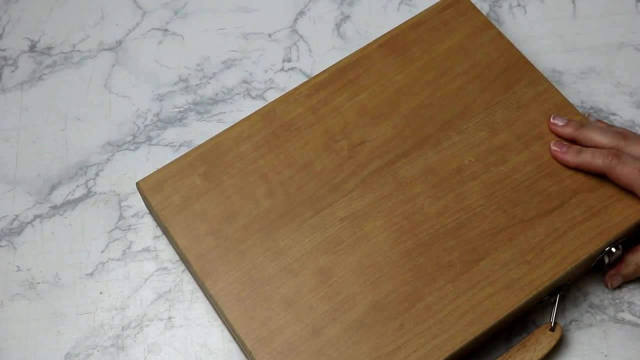 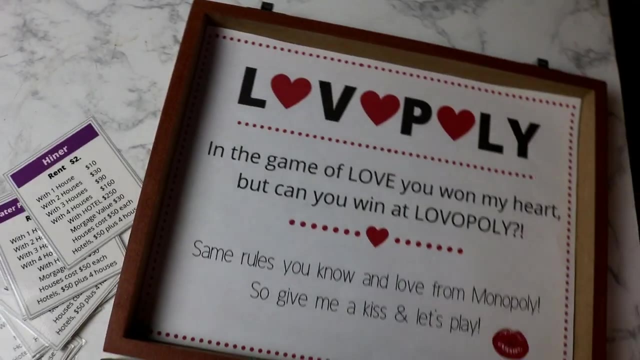 complete little Monopoly set that I can gift him for Valentine's Day. Again, you don't have to do this for Valentine's Day. You can make just one for your friends or your family or whatever, Just as long as it's custom to. whoever you're giving it to and playing it with, they are going to love.